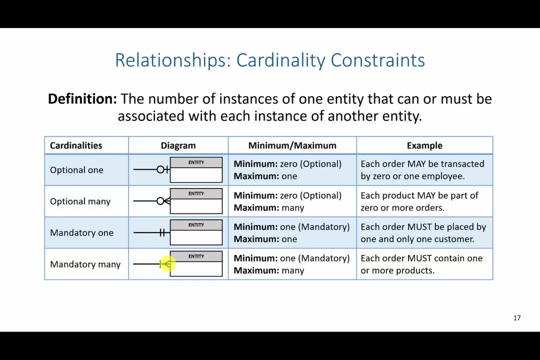 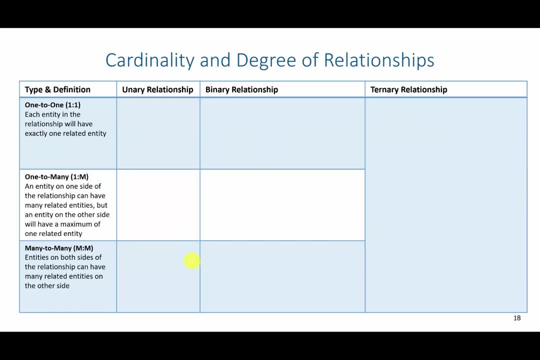 left is going to be associated with at least one, but it could be many instances of this entity here on the right. All right, so now what we're going to do is combine cardinality with the degree of the relationship, So we have three types of relationships that we're going to cover. We have 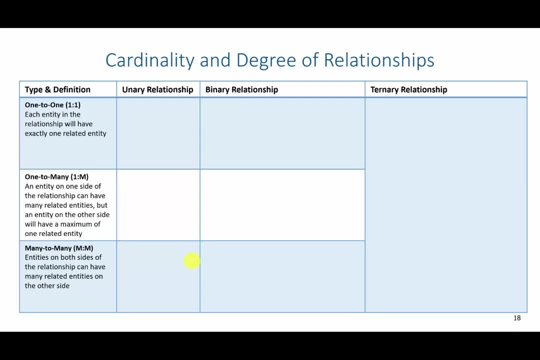 a one-to-one relationship, a one-to-many relationship and a many-to-many relationship. This basically means that we're going to have a one-to-one relationship and a many-to-many relationship. This basically implies the total number of instances of each entity involved. 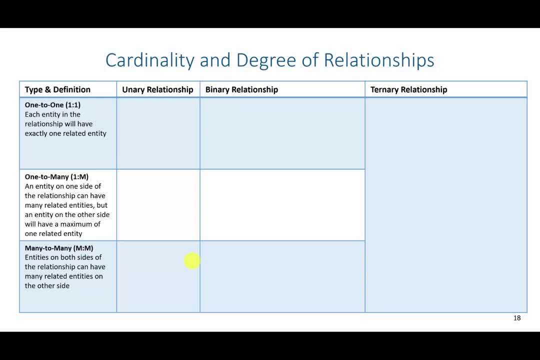 in the relationship and how many that are connected between the entities involved. For example, let's look at an unary one-to-one relationship. So with an unary one-to-one relationship, this person is married to zero or one other person. This means that they. 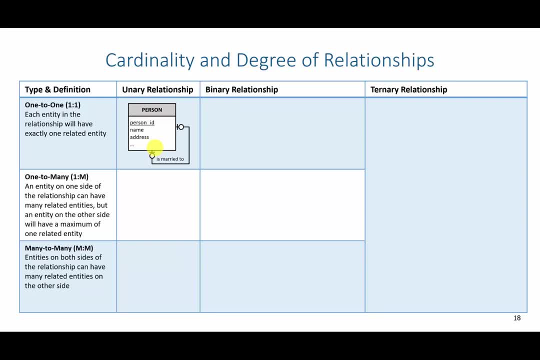 can be single or they can be married, but if they're married, they're only married to one other person. That same person could then be married to zero or one other person In an unary one-to-many relationship. take, for example: we have an employee that could manage. 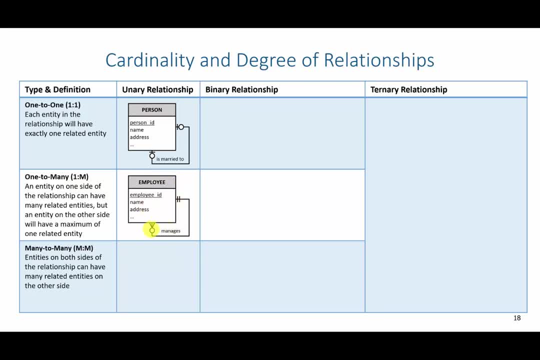 other employees. So this employee can manage zero to many other employees and each employee is managed by one and only one other employee In an unary many-to-many relationship. we have an item contains zero to many items and that item could be contained inside of zero to many items. 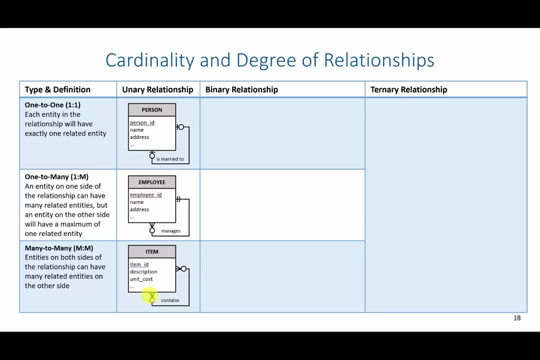 So take, for example, a bicycle. It could contain multiple items: it contains wheels, it contains handlebars, it contains gears, it contains spokes, it contains pedals, etcetera. In a binary, one to one relationship, we have an employee. 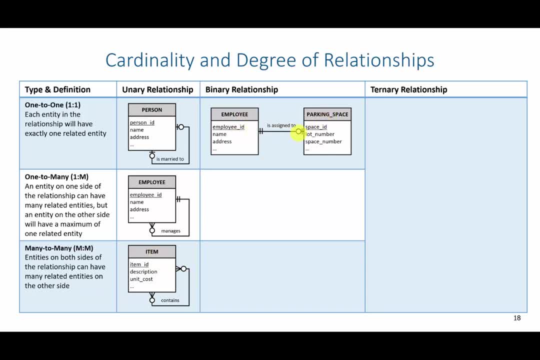 that is assigned a parking space. So an employee is optionally assigned one parking space, but if they're assigned a parking space, they're only going to be assigned to one. However, each parking space is going to be assigned to one and only one other employee. 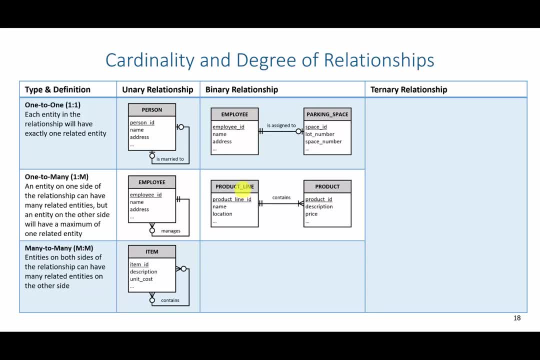 For a binary one-to-many relationship, we have a product line, which is basically the assembly line for producing products. A product line contains one to many products and a product is produced on one and only one product line. In a binary many-to-many relationship, we have a student who can register for one-to-many courses and a 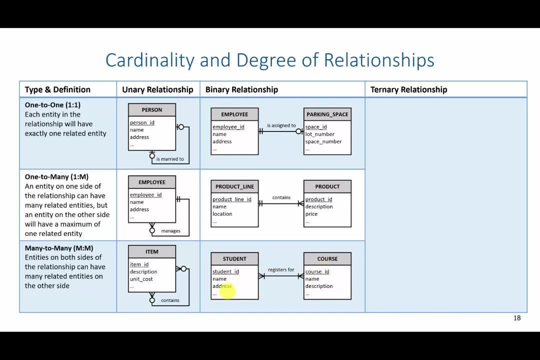 course has one-to-many students enrolled in it. For ternary relationships, we're going to be dealing with many-to-many relationships. For anything with three or more entities involved, we're going to be dealing with many-to-many relationships. So I decided to just merge these cells, but note that this is a 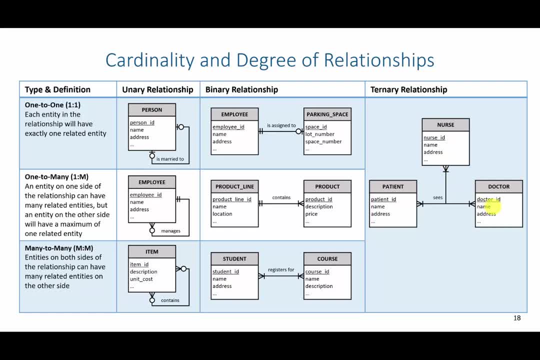 many-to-many relationship indicating that a patient sees a nurse and a doctor all at an appointment, and so we could have: a patient could see many nurses, a patient could see many doctors, a doctor could see many patients, a doctor could have many nurses that help them during their appointments, etc. Additionally, each 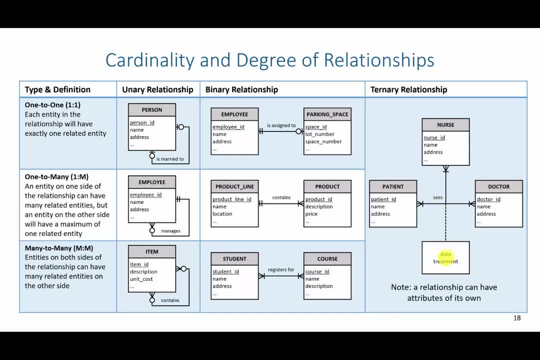 relationship could have attributes of a their own. So for this appointment that we're calling it, it could have a date and a treatment. Now, this date is not associated with the patient nurse or doctor, neither is the treatment associated with the patient nurse or 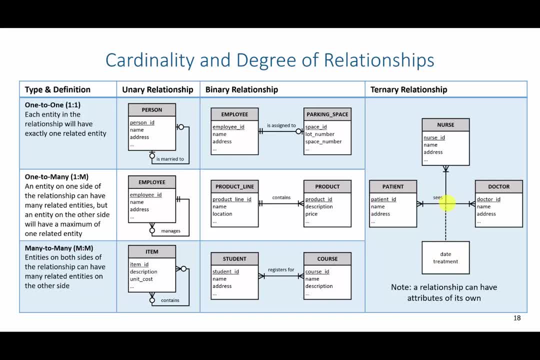 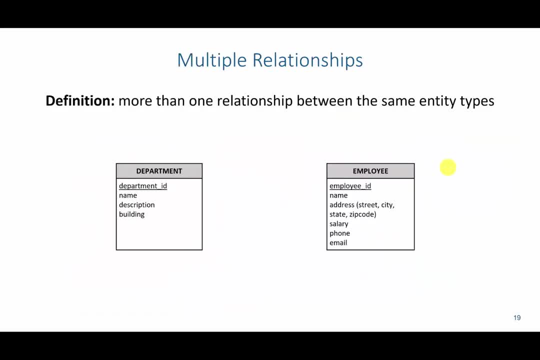 doctor Rather. these exist because of the existence of the relationship between patient, nurse and doctor. Additionally with relationships, we can have multiple relationships between one or more entities. So, for example, a department has one-to-many employees, an employee works in one-and-only. 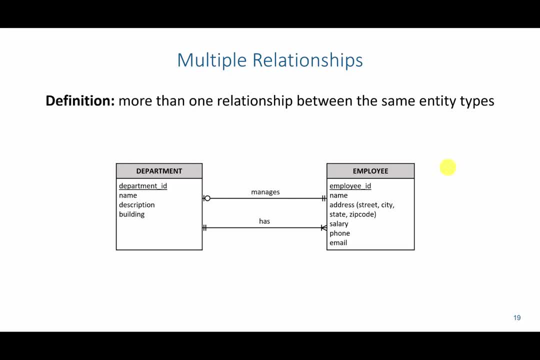 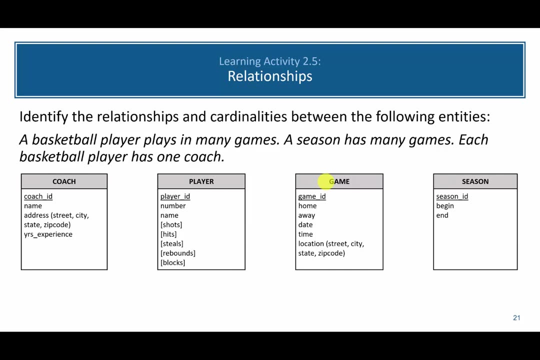 one department. Additionally, an employee could manage that department. So we could have one employee manage that department, but each department is managed by one and only one employee. So let's use the learning activity we discussed previously and we are going to then identify the relationships and 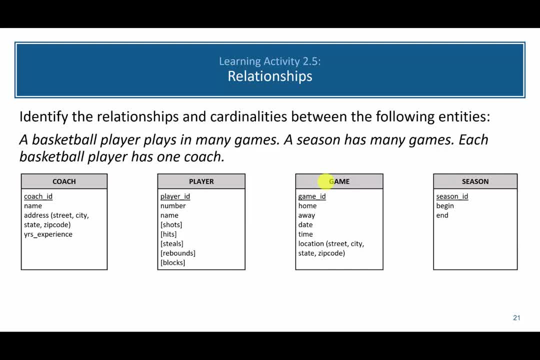 cardinalities that would exist between these four entities that we previously identified. So go ahead, pause the video, try this on your own and then come back to compare your answers. Alright, welcome back. So we see here. this first sentence says: a basketball player plays in many games. So a player plays in many games. So 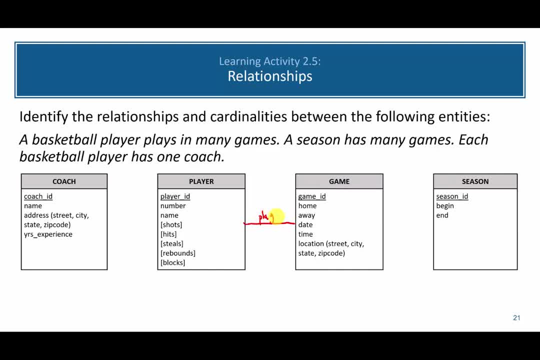 that's the relationship. The relationship type is going to be the verb, so we're going to say plays in many games. So all we know from that sentence is that a player can play in many. so there's the maximum against game. Now this is where 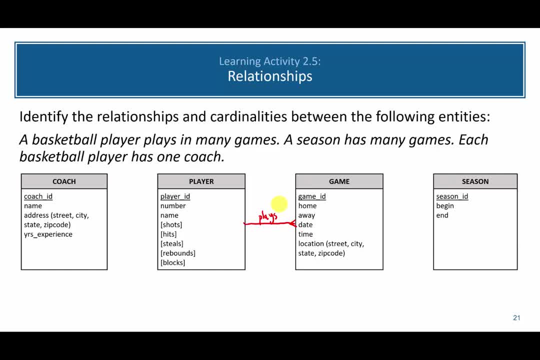 you have to make some assumptions. Maybe you're not given all the information you need. but does a basketball player have to play any games? No, they could just be a benchwarmer. So we could just say this is an optional relationship on that side. Now a game. 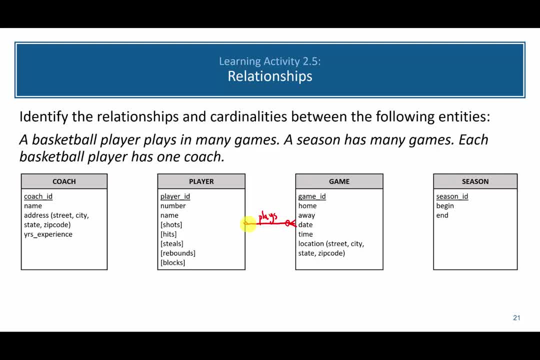 has at least 10 players, but we're going to just represent that as a mandatory many, So obviously there's going to be more than one, and in some notations what they do is in order to have a game, you need to put a number under there. 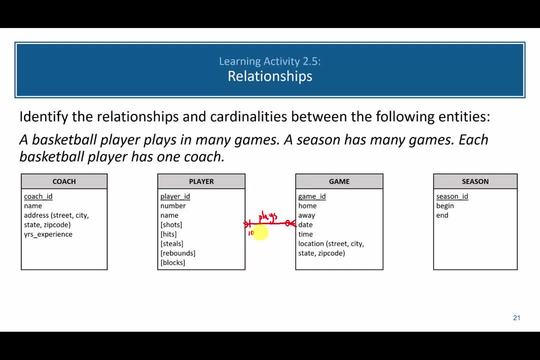 representing that this line is not actually one, but it is 10.. So, but we're not going to do that, We're just going to have a one to many here. Alright, let's go to the next sentence. A season has many games, So a season has many games. Now does a season have to? 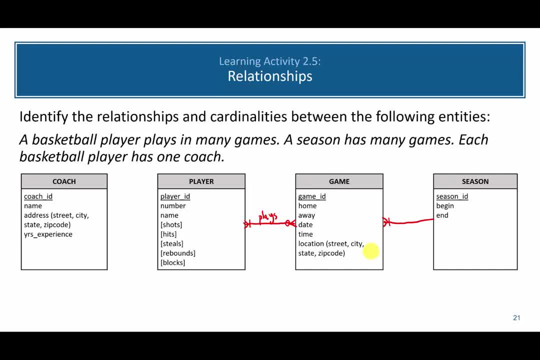 have at least one game. Yes, so we're going to say it has one to many games. Now, a game can be in how many seasons? The game can be in one and only one season. So we'll just go ahead and put the verb here of has, because that's what. 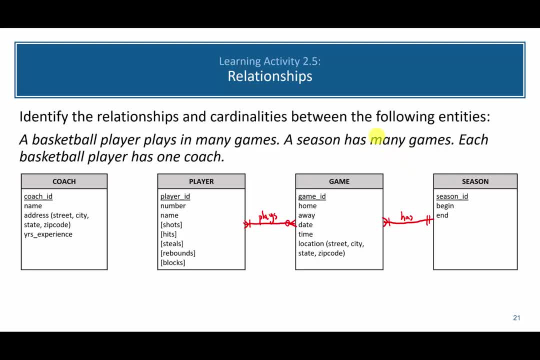 we have in that sentence. Alright, this last sentence says: each basketball player has one coach, So a coach coaches players. So let's go ahead and write that in, All right, so a coach could coach one to many players and a player could be coached by. this is something you're going to have to consider. Is it multiple? 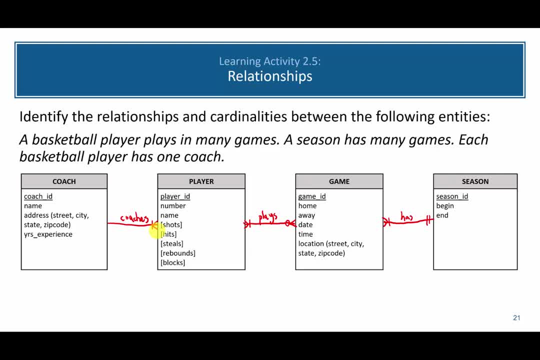 coaches. Is it one coach? Is a coach and assistant coach different, or are they the same? I'd argue the same. You just put an attribute of type into the coach entity to represent that, Based on that assumption that a player could have multiple coaches, we would just draw a line here saying a: 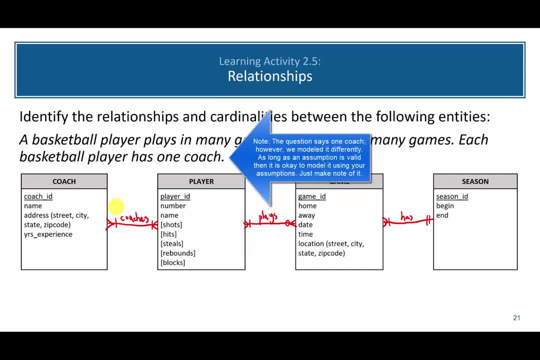 player has at least one coach, but they could have many coaches that coach them.